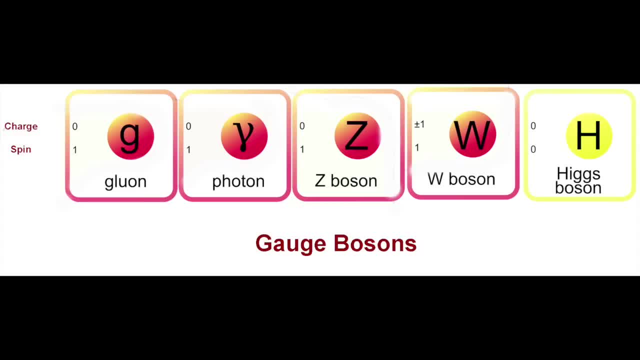 the strong interaction or strong force. The exchange of gluons between quarks binds them together so that they can form larger particles such as protons and neutrons. Photons are the force carriers of the electromagnetic field. W and Z bosons are the force carriers which 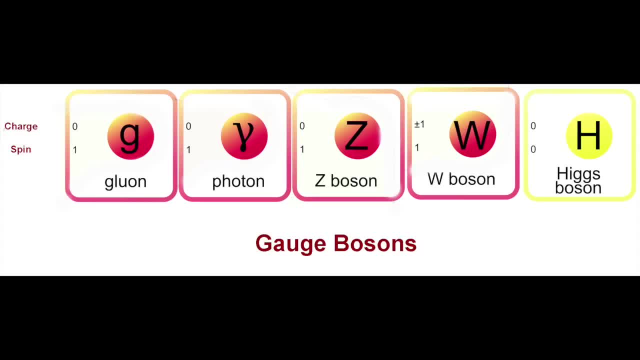 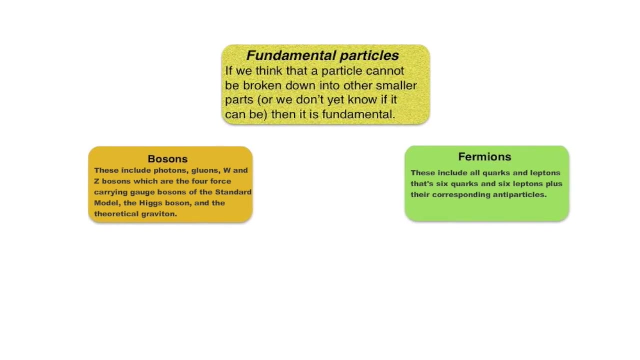 are involved with the weak force. The interaction of these bosons with the Higgs or the Higgs field is responsible for their mass. The Z, W and Higgs bosons are far more massive than any of the fermions, than any of the quarks or leptons- The names of the fermions might be more familiar. These: 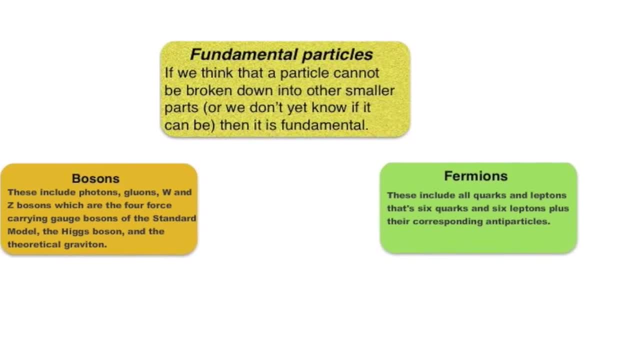 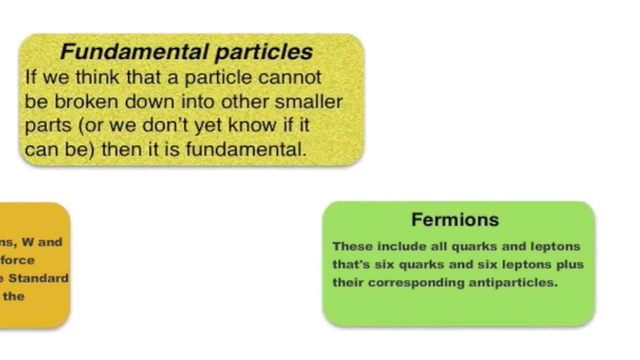 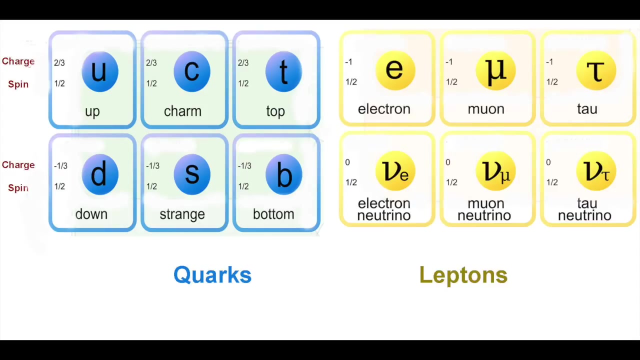 are all of the quarks and leptons. A link at the end of this video and in the information below will take you to quarks and leptons for beginners. There are 24 quarks and leptons all together. Most importantly, there are the up and down. 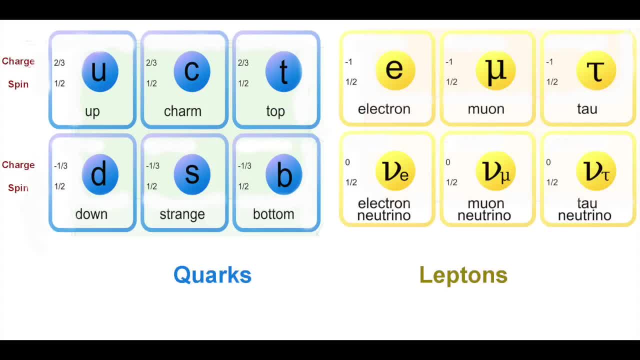 quark and the electron and neutrino Combinations of the up and down quarks produce neutrons and protons- Two downs and one up for a neutron and two ups and one down for a proton. Electrons are fundamental parts of all atoms. This is one of the things that makes the quark and 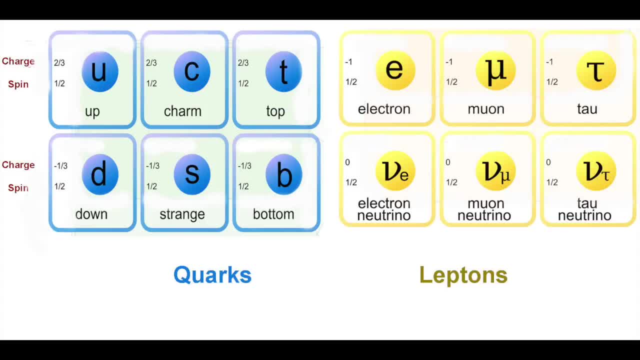 neutrons, so important to us, occupying energy levels surrounding the nucleus. Neutrinos, pervade the Universe, streaming out from our Sun. as a consequence of all nuclear actions and reactions. Every one of these particles has an antiparticle, and that's why there's 24.. 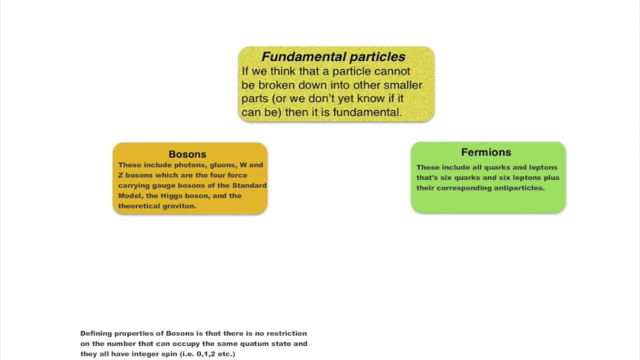 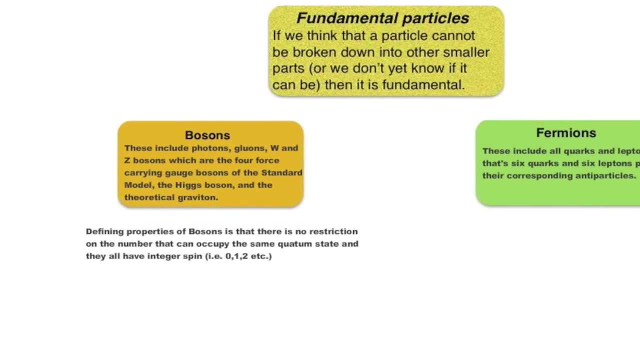 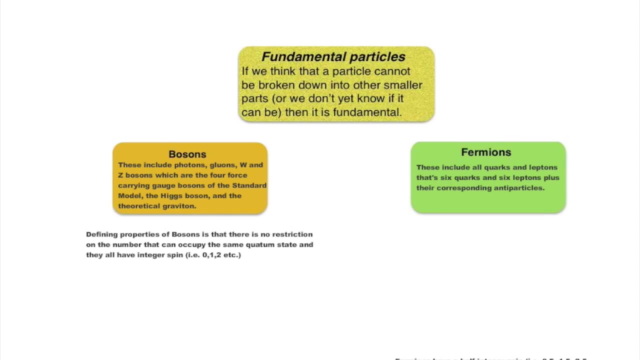 Defining property of bosons is that there is no restriction on the number that can occupy the same quantum state at the same time and they all have integer spin, that is 0,, 1,, 2, and so on. All fermions have half integer spin, that is a half, one, half, two, half, and so on. 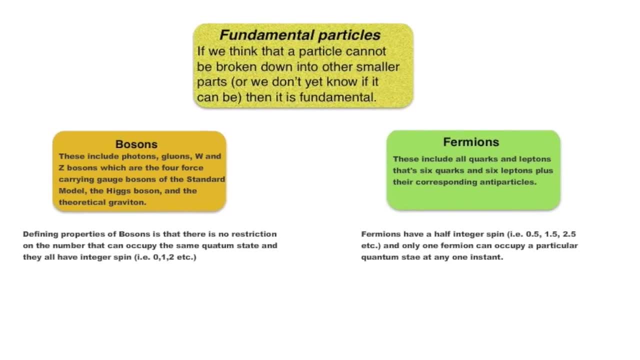 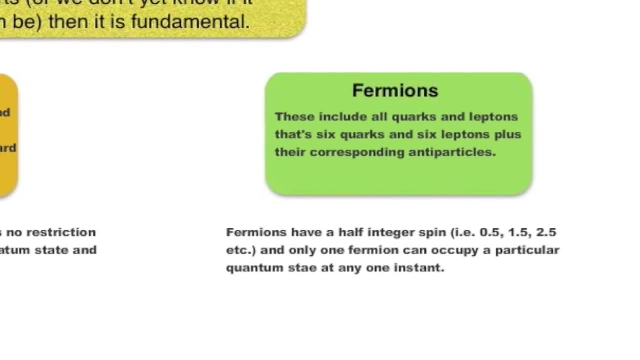 In addition, only one fermion can occupy a particular quantum state at any given time. If there's more than one in the same space, then at least one property of each fermion, such as its spin, has to be different. Going back to the question,